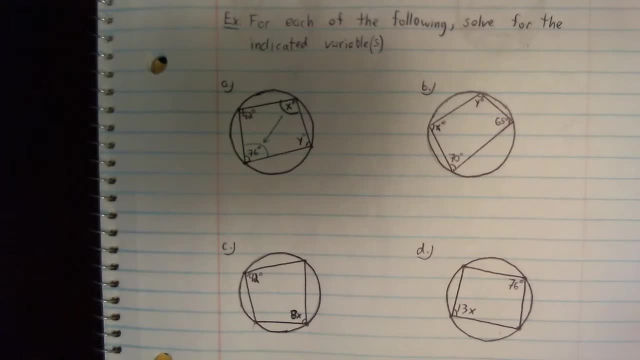 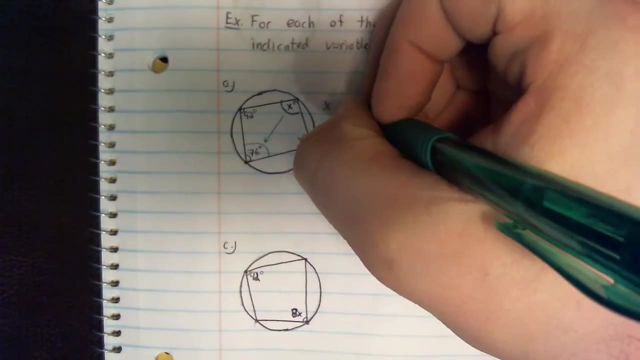 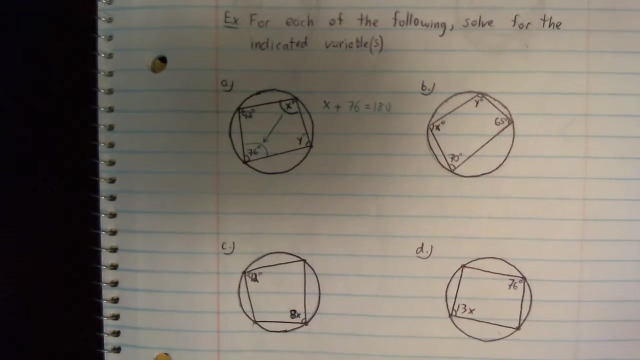 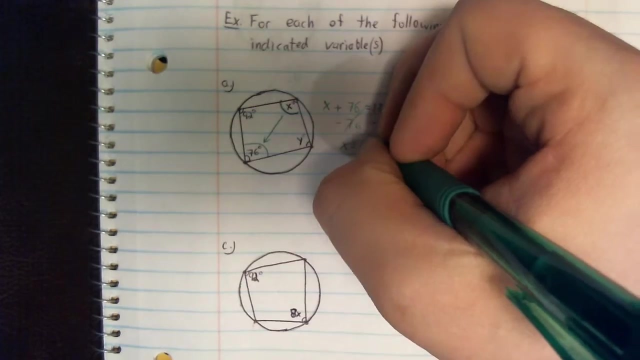 Do not choose blue, Do not choose egent. simple statement that means to useeger. you're going to lose them. So, on the independence statements, what you're going to do is add exact amounts of x to your plot. And now let's take a look at. 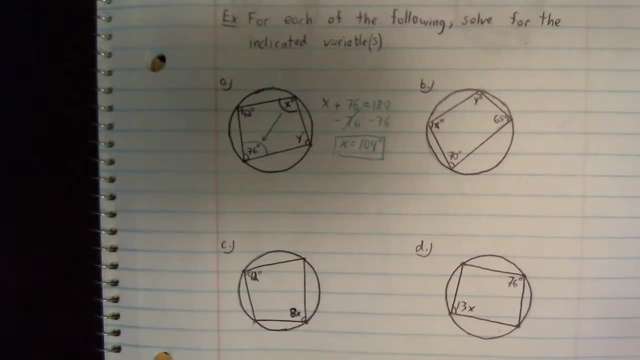 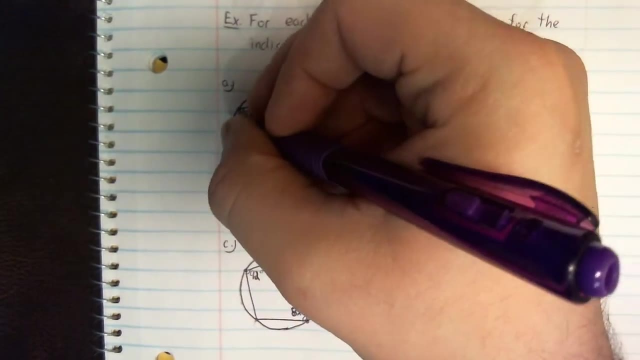 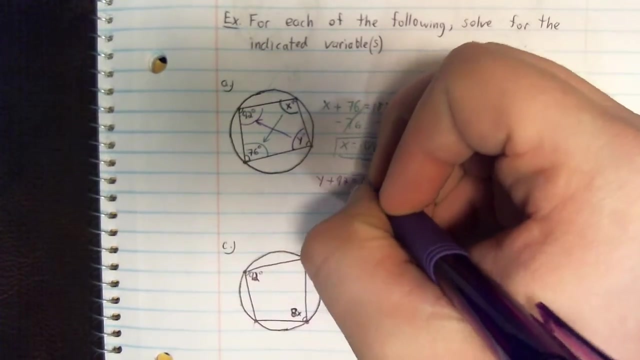 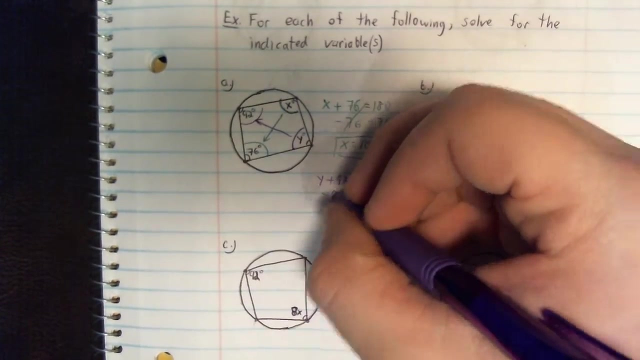 degrees. I'm going to do angle Y in purple. Here's angle Y Again, the angle opposite, angle Y, is right here, 92. Remember that we're going to be adding these two together and setting them equal to 180 because they're supplements. Subtract 92 from both sides, That leaves us with 88 degrees. 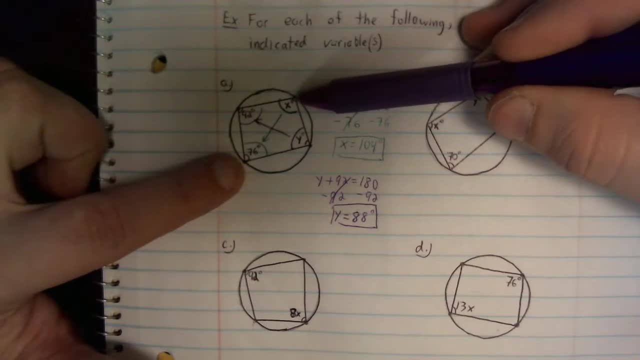 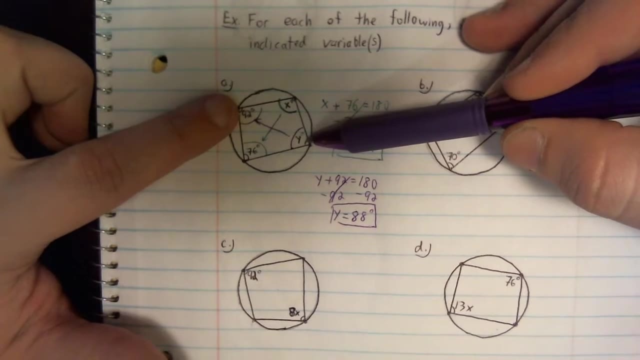 Okay, so we found angle X to be 104.. Remember that they're supplements. They should add to 180.. We found angle Y to be 100.. I'm sorry. We found angle Y to be 88 degrees. Remember these two. 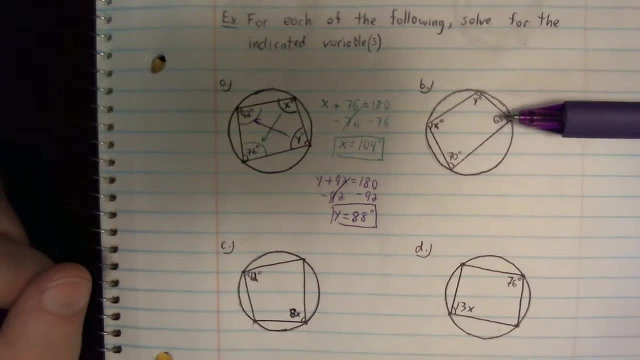 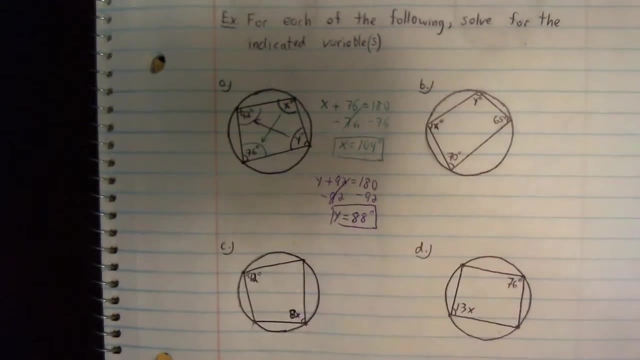 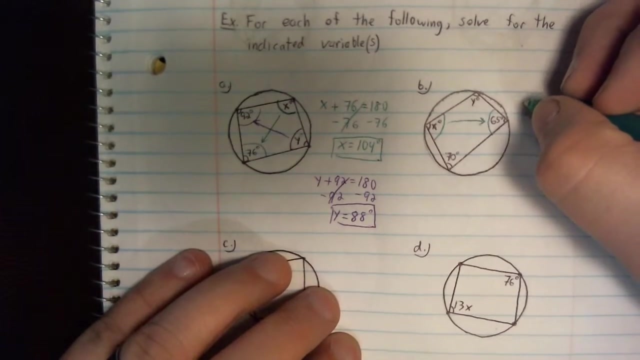 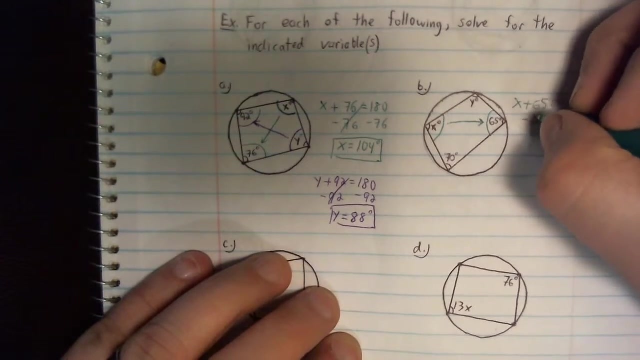 angles should add up to 180.. Okay, so again, if you'd like to try any of these ones out on your own, go for it. Let's test this next one. Angle X is opposite of 70.. Angle Y is 65 degrees. So we would say: X plus 65 equals 180.. If you want to subtract 65 from both, 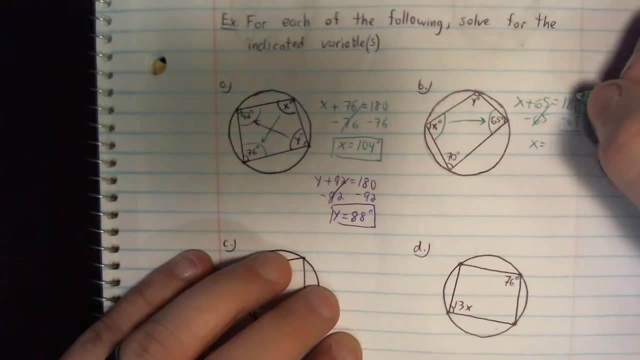 sides: 180 minus 65.. That's going to be 115 degrees. Okay, All right. And angle Y is also opposite of 70.. All right, Angle Y is opposite of 70.. All right, y is opposite of 70.. 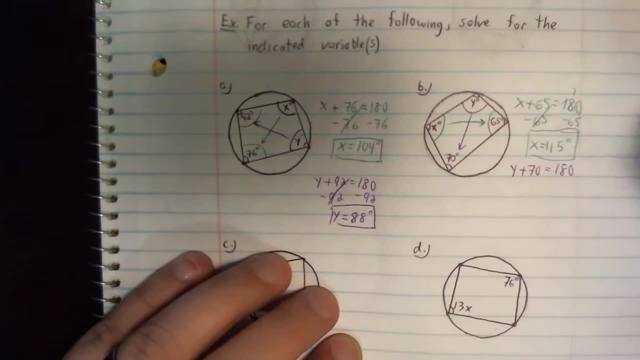 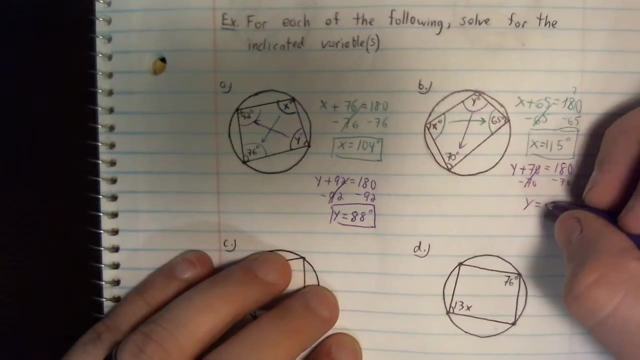 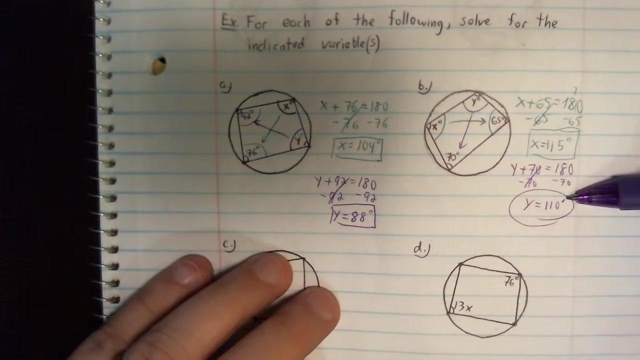 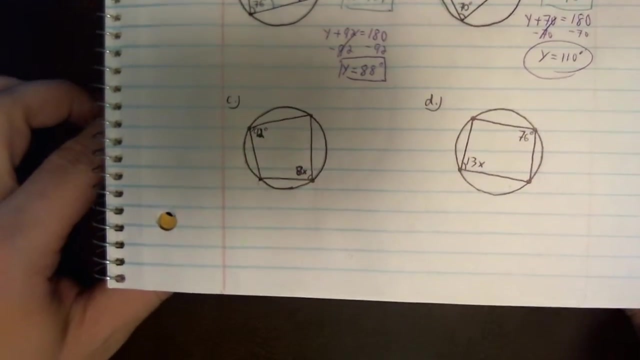 So y plus 70 will add to 180.. Subtract 70 from both sides, that gives us 110 degrees. So we found x to be 115 degrees, y to be 110 degrees. Remember these angles are supplements when they're opposite of each other. 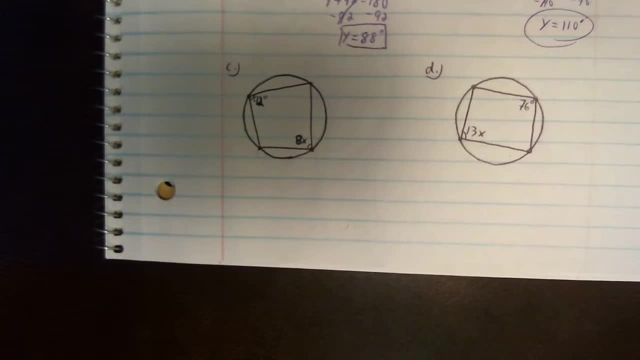 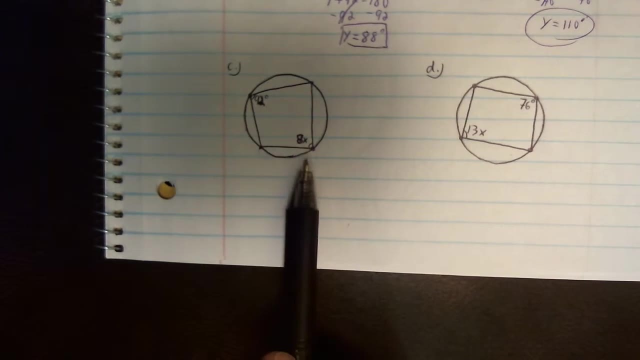 So when you look at the next two problems, they don't give you quite as much stuff to solve for. I'm sorry if this is a little bit blurry. This is 92 degrees, This is 8x. So if you'd like to try these out on your own, 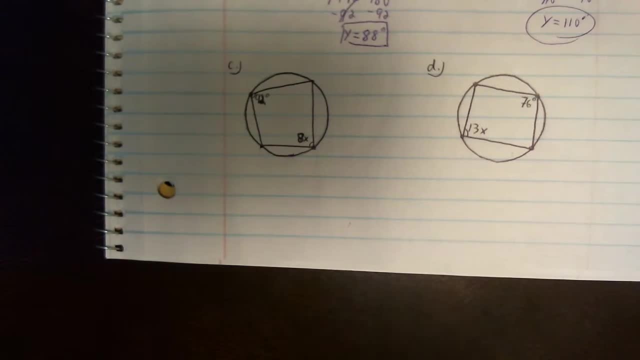 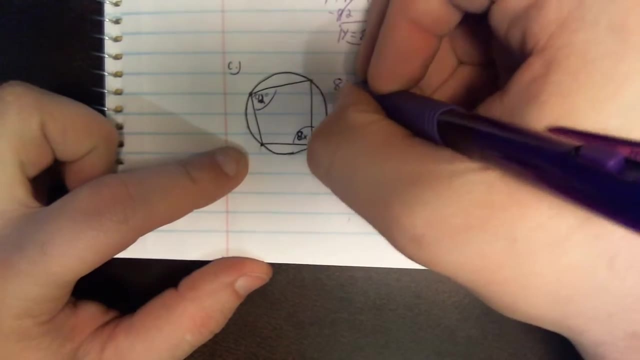 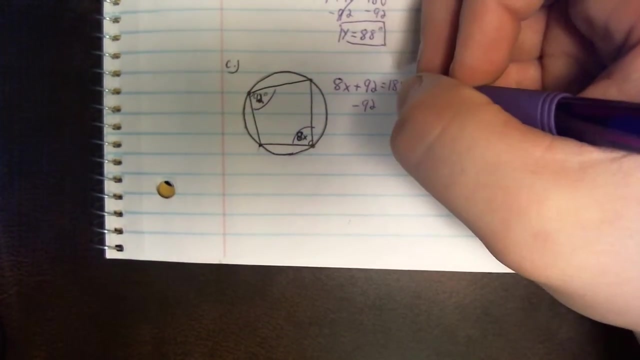 now you know what those numbers are, So let's test it. We know that these two values have to add up to 180.. So 8x plus 92 equals 180.. OK, I'm going to divide. I'm sorry, I'm. 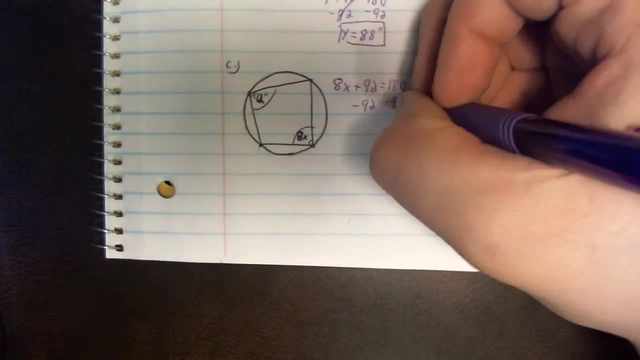 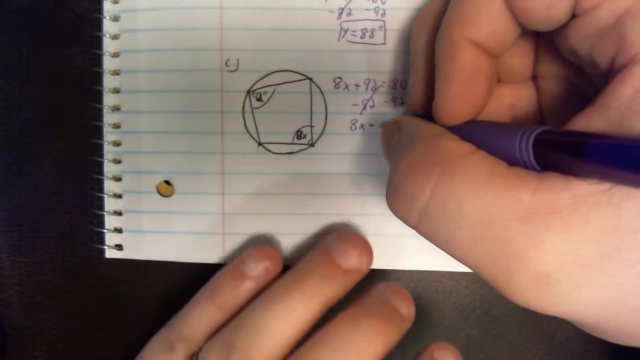 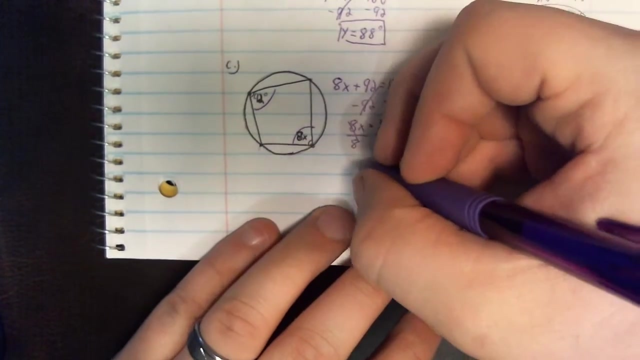 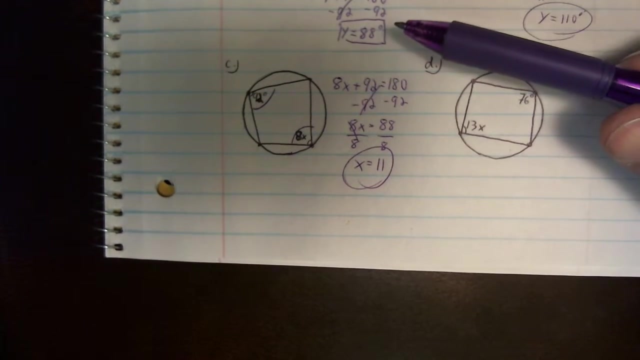 going to subtract 92 from both sides. So 180 minus 92 leaves us with 88. And once we divide by 8 on both sides, we get x equaling 11.. That's all that they asked us for. Notice real quick before the values that we were finding. 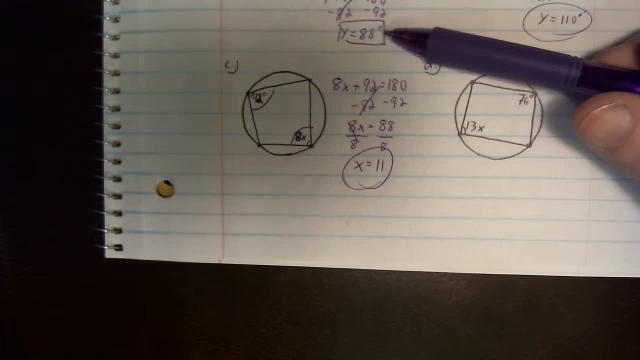 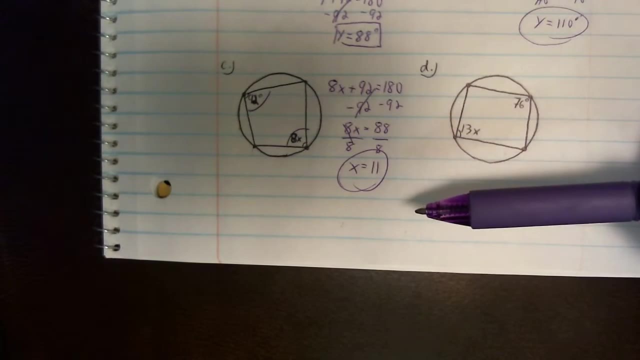 were just 1x. That's all they asked us for. Notice real quick before, the values that we were finding were just 1x. The drop-down bar numbers: just give us the number eight, because it was exactly the same. 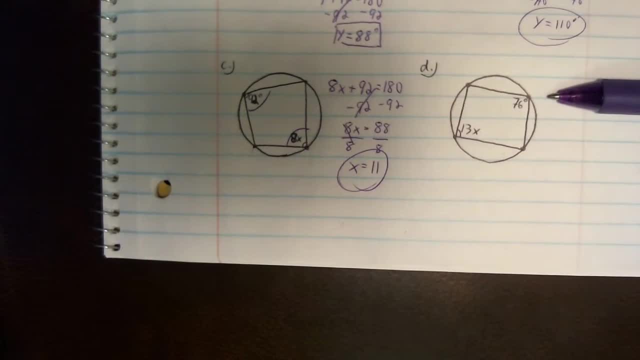 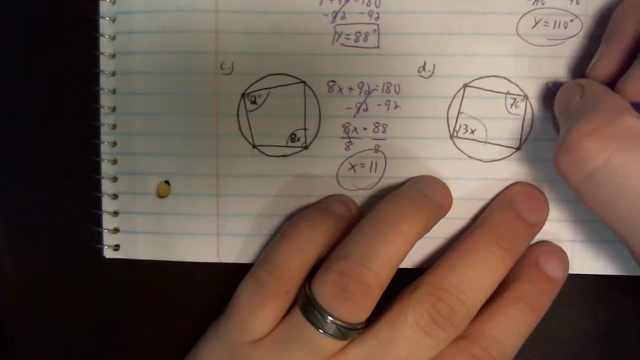 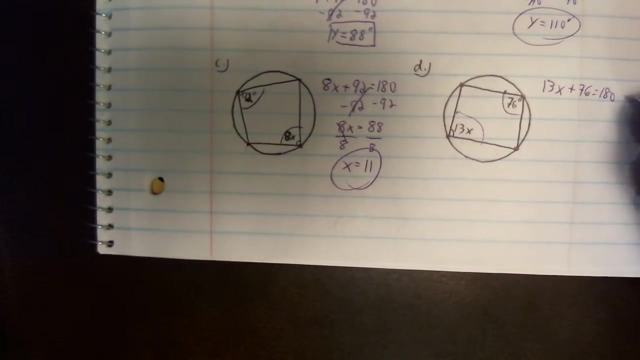 And yet this one entry is что It's thought to be, that one entry, That is, it's helping to separate those side divisors. But, student, no, I said that's what they asked us for. equals 180. we're going to want to subtract 76 from both sides. that leaves. 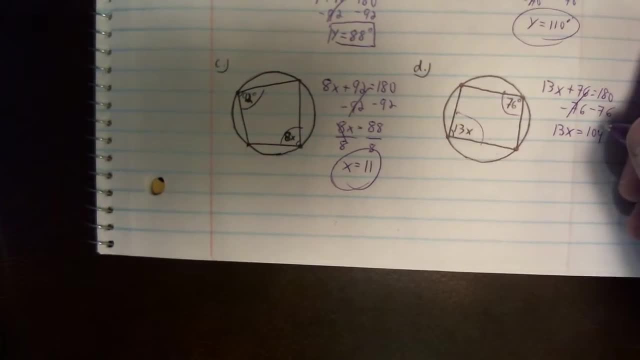 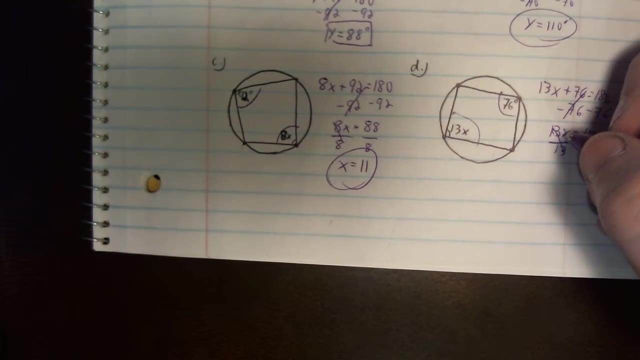 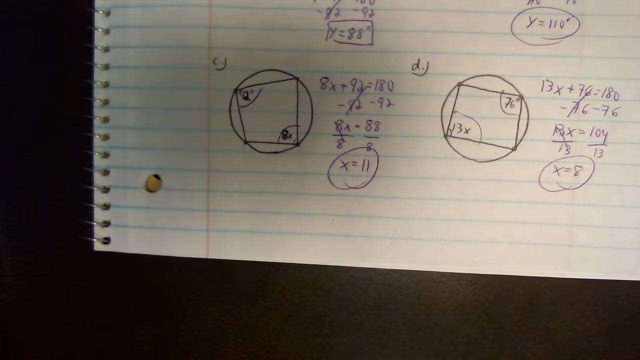 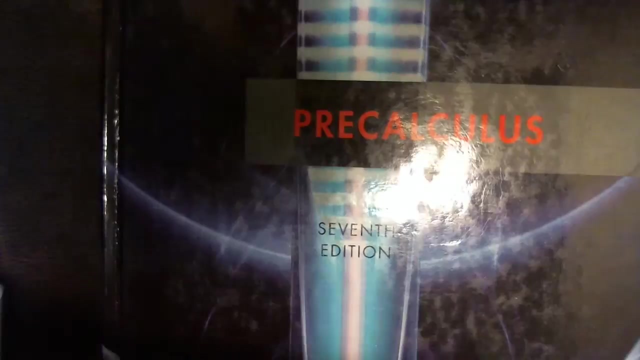 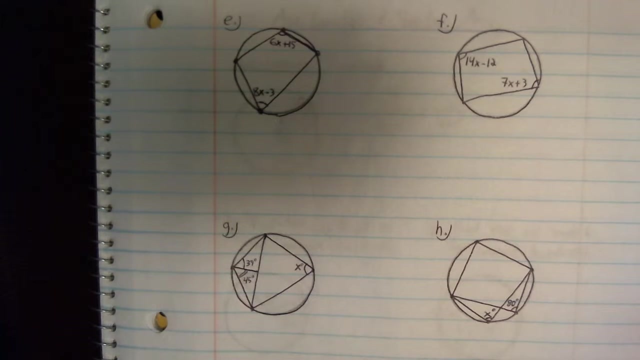 us, with 13, X equals 104, and then we have to divide by 13. so we divide 104 by 13 and we get 8. a pretty simple, pretty easy. a few more problems to look at. again, all of the process to these problems are going to be the same. so if you want to, 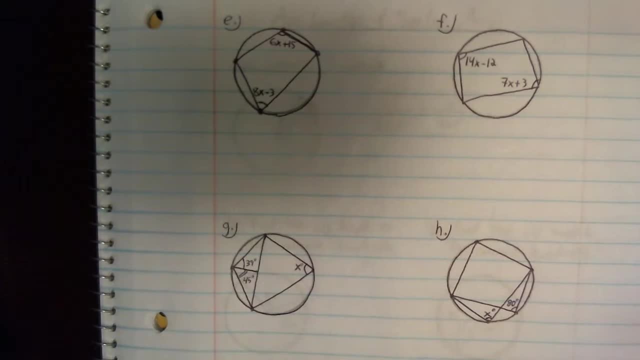 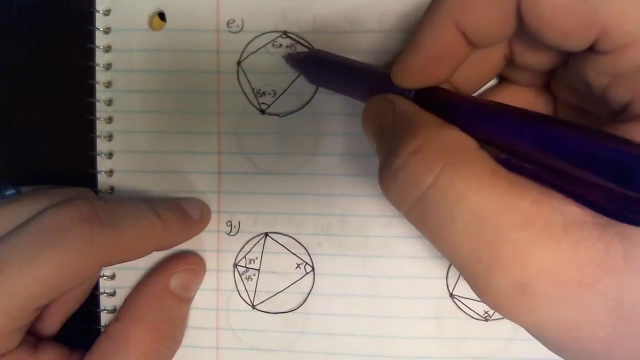 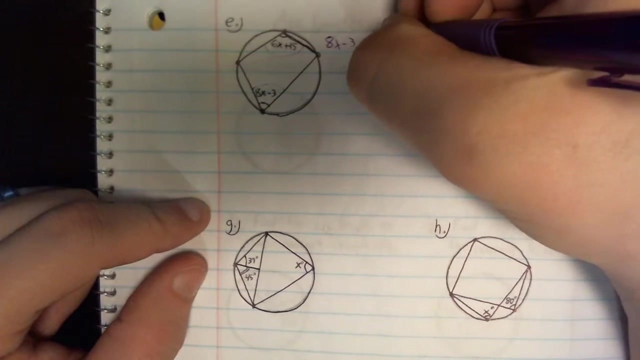 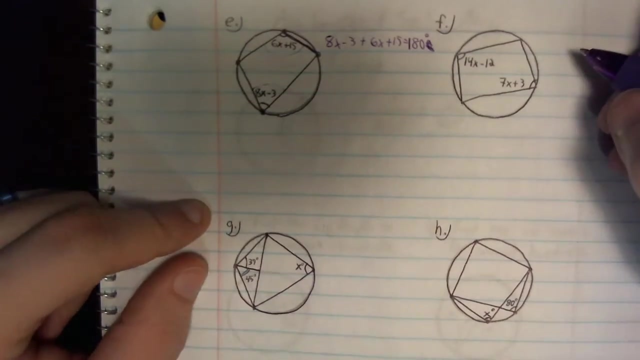 test these ones out. try them, see how you do. it's worth a shot. right, the angles in question here: 8x minus 3 and 6x plus 15. they're going to add and they're going to be equal, oops, to 180 degrees. okay, so let's combine like terms. 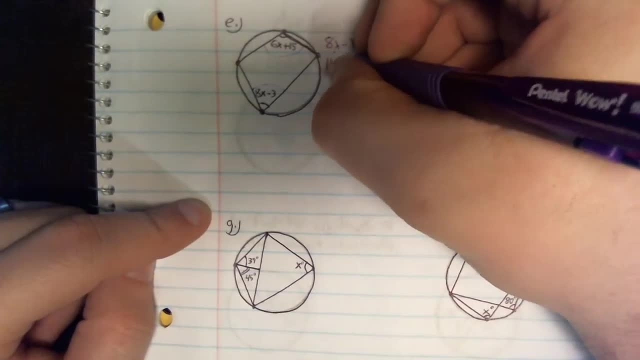 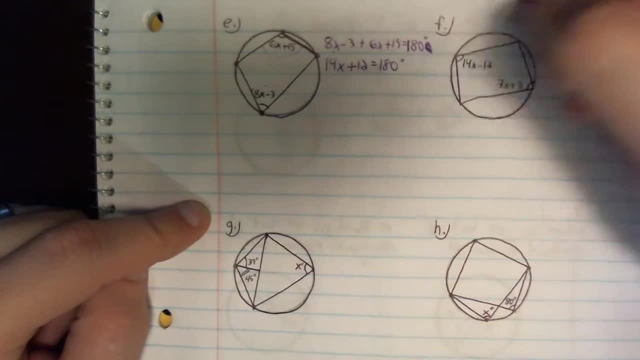 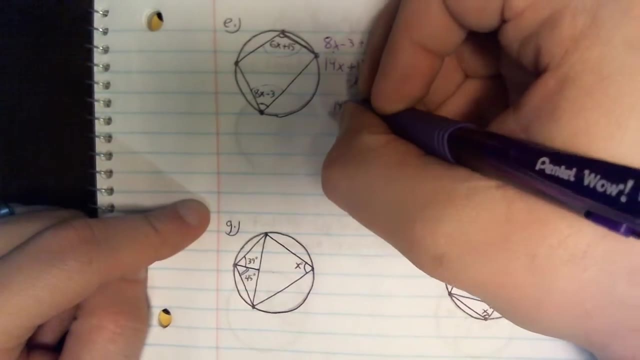 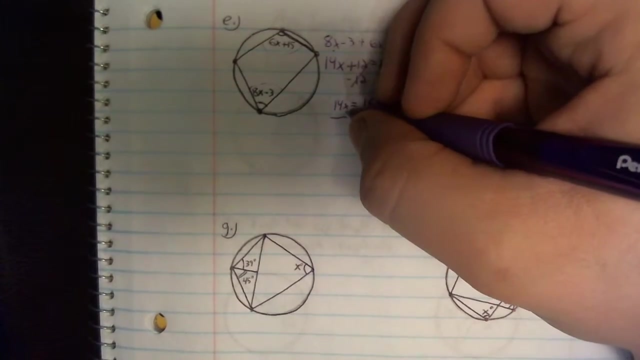 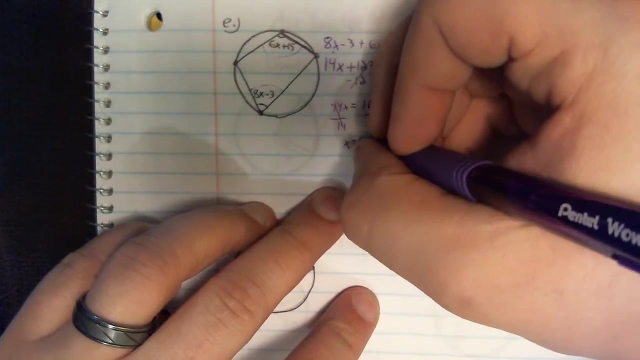 that's 12, and we got 180. on the other side, we're gonna subtract away 100, I'm sorry. we're gonna subtract away 12 from 180. that's gonna give us 168. and then we need to divide both sides by 14. that gives us X equaling 12. 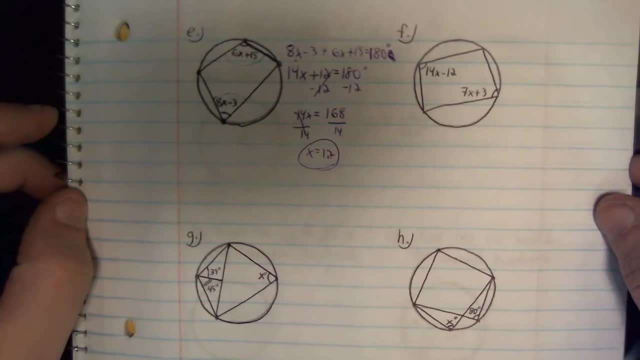 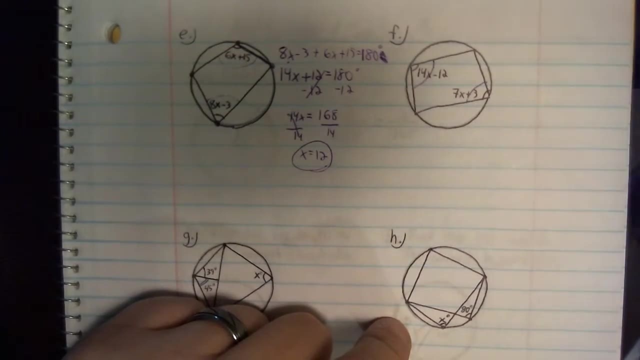 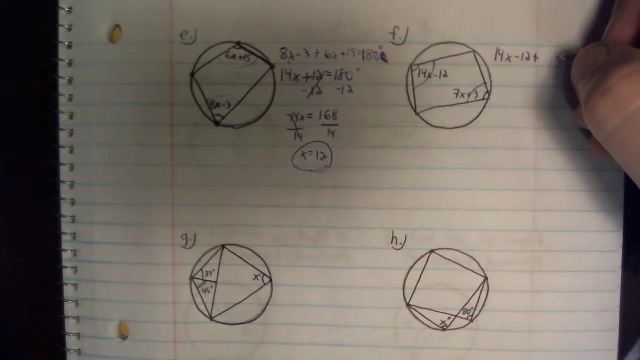 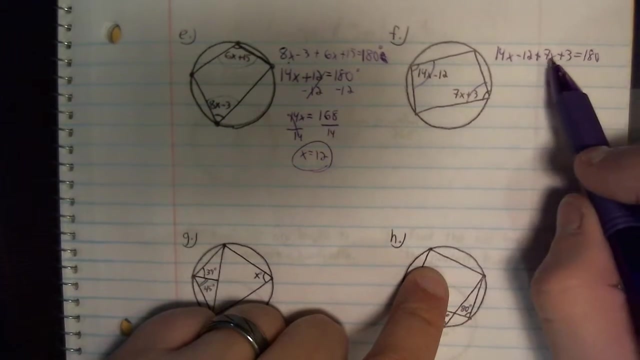 aligned with 14, which is 4. welcome to population. okay. problem F: remember that those angles are opposite. that means they add to 180: 14x minus 12 plus 7x plus 3 equals 180: 14 X 7 X. that's total: 21: X negative, 12 positive 3. 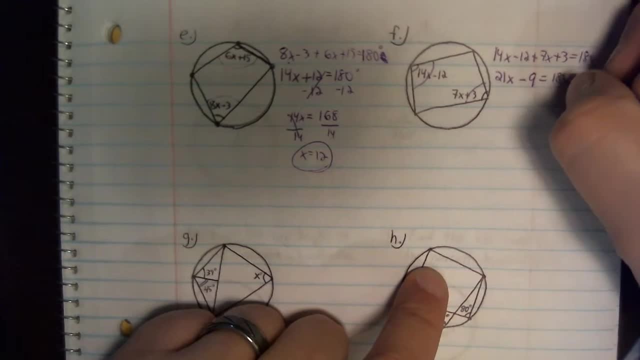 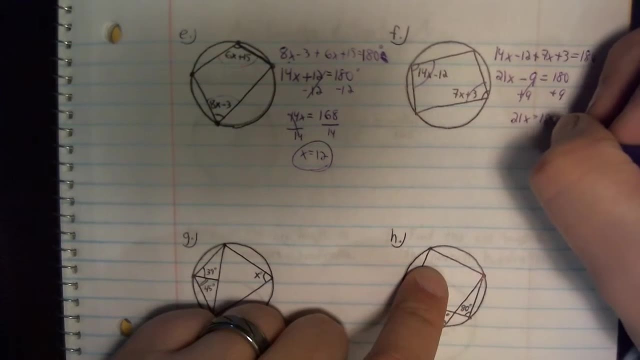 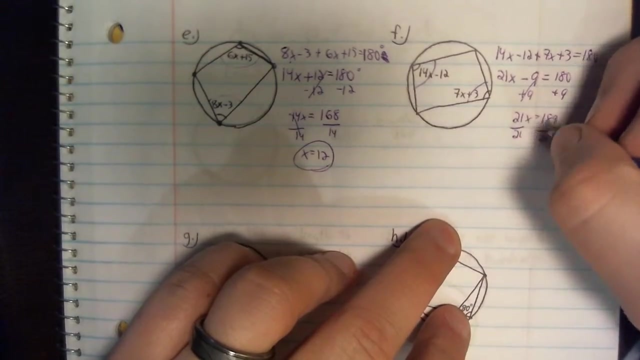 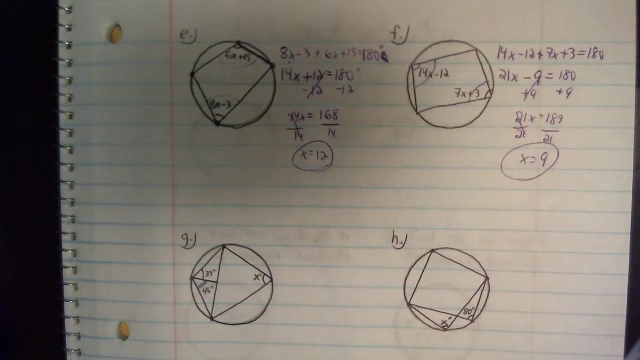 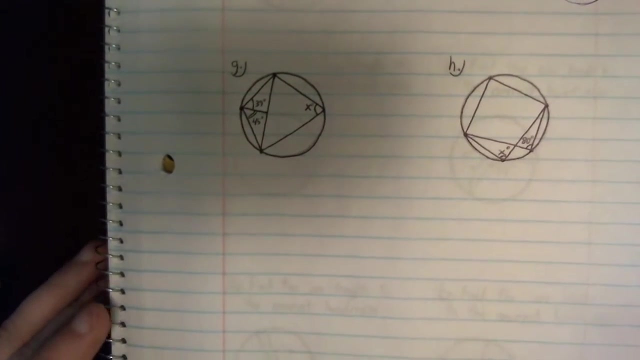 3. that's negative 9. we want to add 9 to both sides and then we have to divide by 21. that gives us a value of 9. hopefully you're doing okay with these. the one more set of problems to go. these ones are a little bit different. okay here. 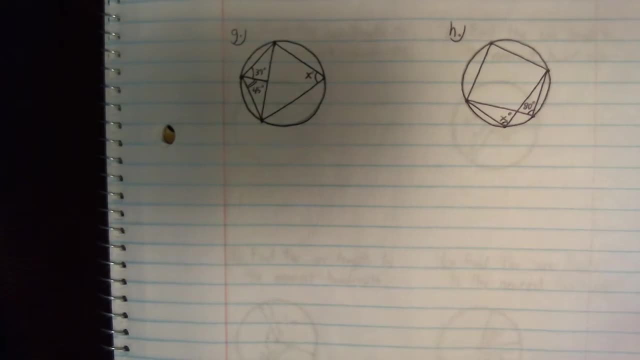 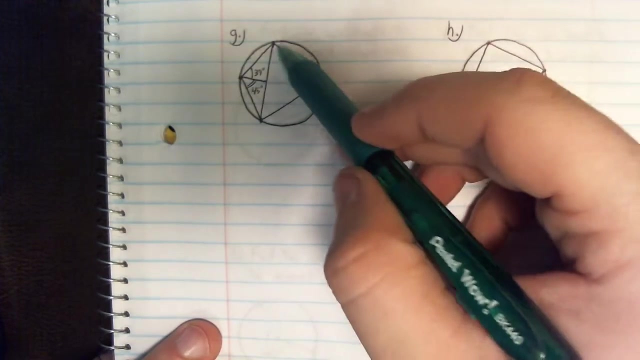 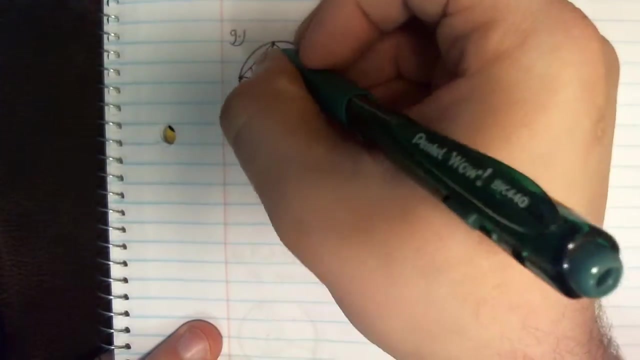 they give you more than just a quadrilateral. right, you might notice that the quadrilateral in question is this entire shape, but they have a piece broken up over here. don't let that fool you. okay, the quadrilateral right here has one angle that's built in to the other side of the quadrilateral and 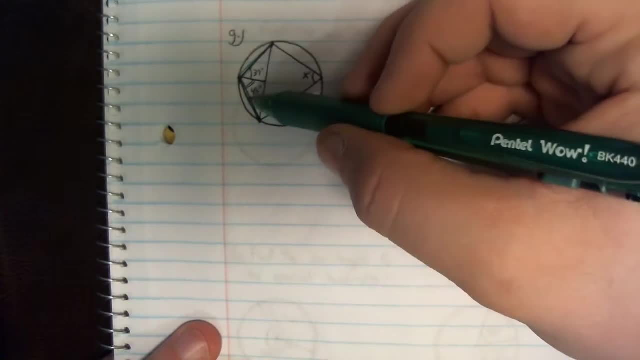 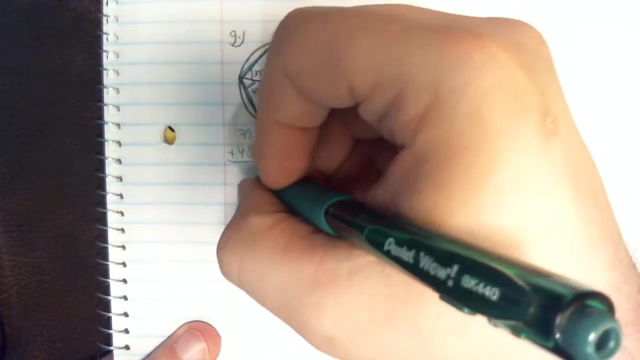 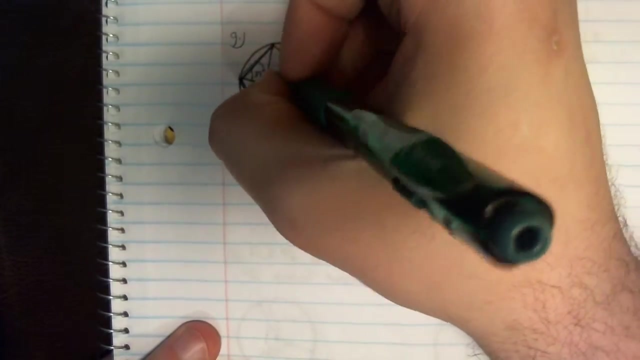 it's built up of two smaller angles, so if I want to know the length of this entire angle, I would have to just add those two values. so if I add 39 and 45, I get 84 degrees. well, now that I know what that angle is, here for this entire. 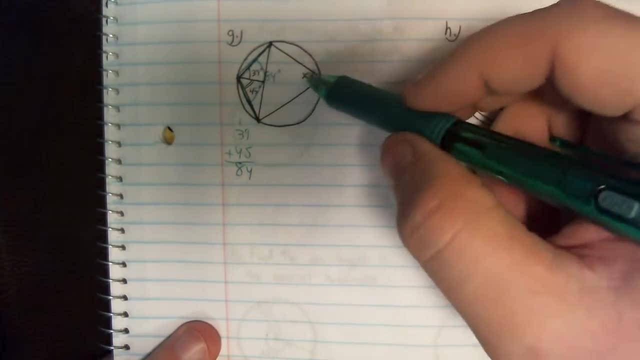 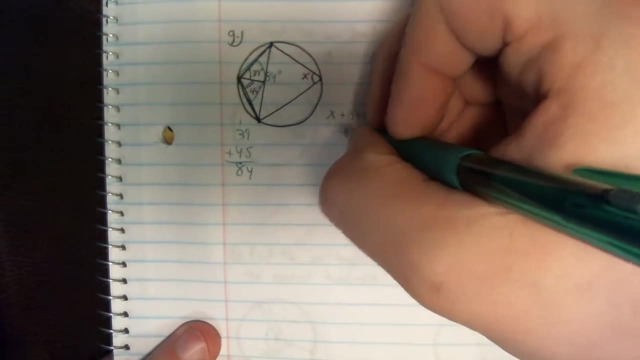 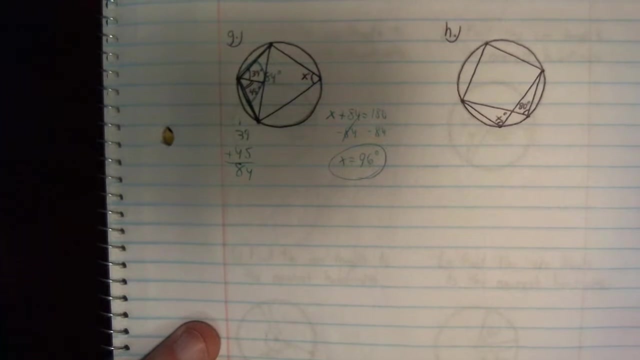 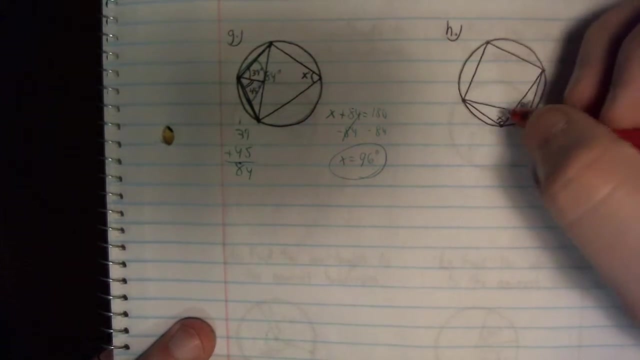 quadrilateral angle. I know that these two opposite angles must be supplementary, so I just add: plus 84 equals 180 will subtract 84 from both sides. that'll leave us with 96 degrees for X, okay, and as far as H, again, don't let this bother you. here's one of 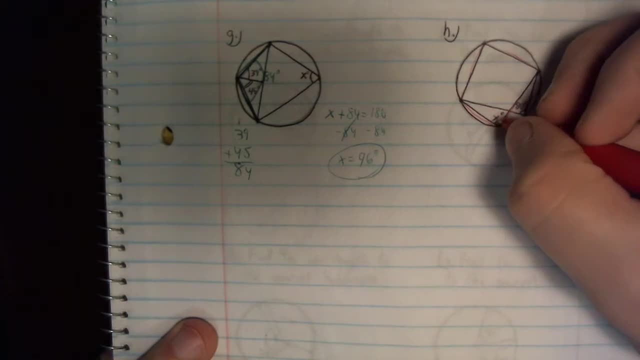 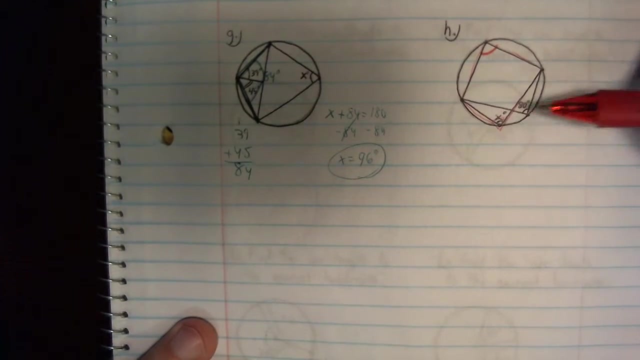 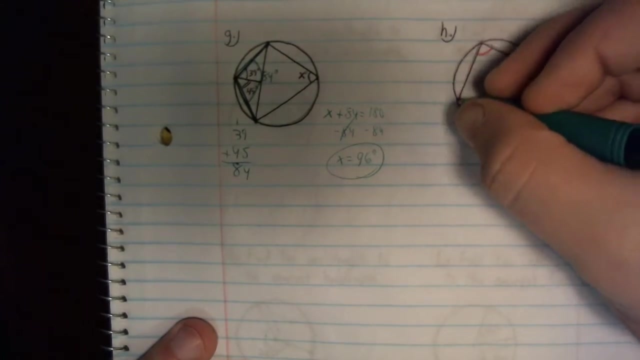 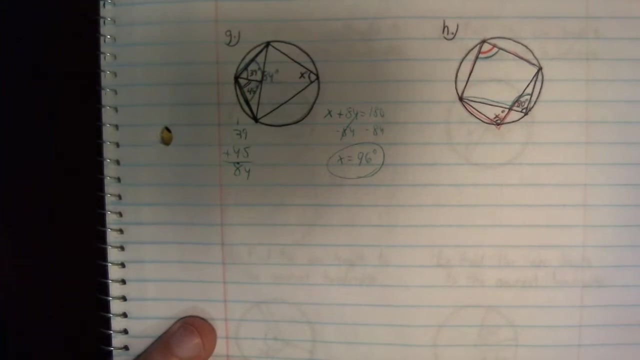 the quadrilaterals. here's X. here's the angle opposite of X. well, we don't know that value, so we can't really find X right now. however, we do have another quadrilateral. they gave us an angle here of 80. the angle opposite of it is right here, which is- hey look, the same angle.